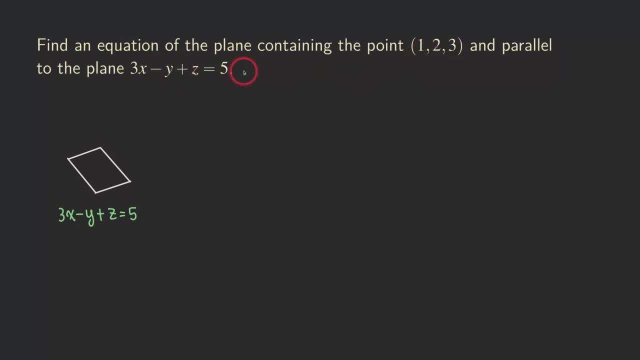 that this point is not lying in this plane here, because you can just plug in the x, y, z and then satisfy this equation. So we know that the point is just somewhere else. So if you just look at this right here, okay, so this point it's just somewhere in the space. Let's say it's right. 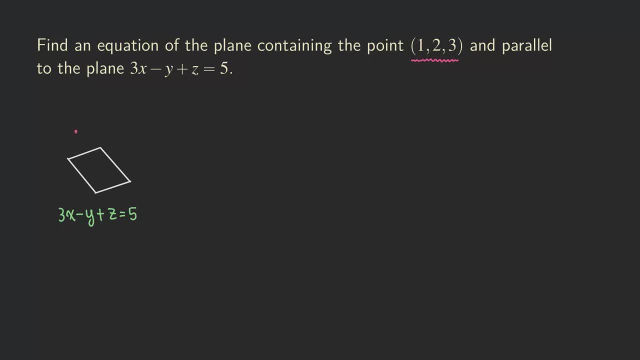 here, for example: Okay, so that's, that's the point, That's this point. So 1,, 2, and 3.. So now the question is: how do we determine another plane that we want so that it will? 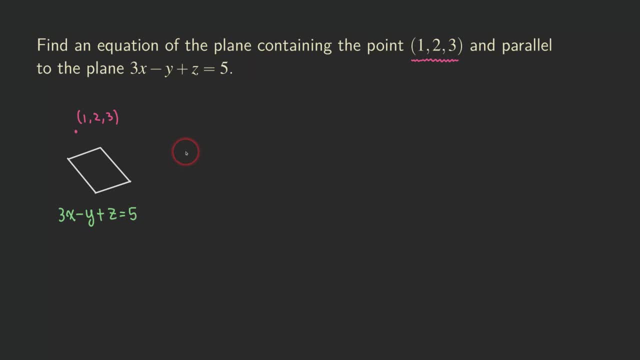 contain this point and also parallel to this plane. So you know that if we are another plane that's contained in this point and also parallel to this plane, right here, the 3x minus y plus z equals 5, right, Then you can see that we're supposed to be drawing the. 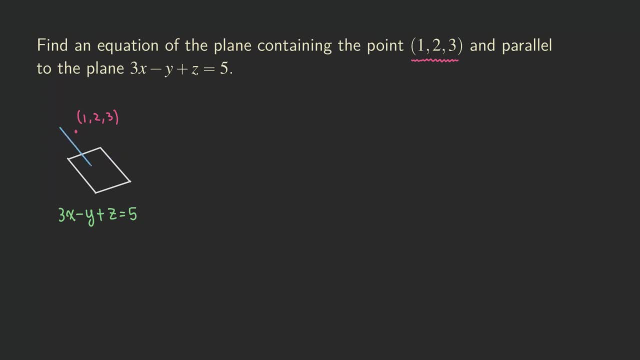 plane like this right. So- and this is again, this is for demonstration, So it's not really accurate. So you can see that this blue plane that we're trying to find. So our goal here is to find an equation for. 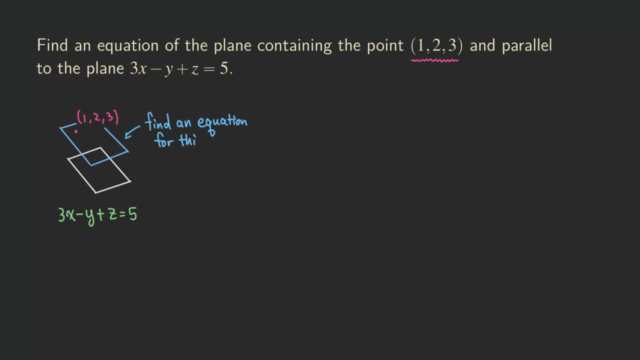 this blue plane here. Okay, and so, and it contains this point, And then you can see that when you draw the normal vectors for both planes, okay, so when you draw the normal vectors, then do you realize that we can actually say that the two normal vectors are parallel to each other. Okay, so the one for the 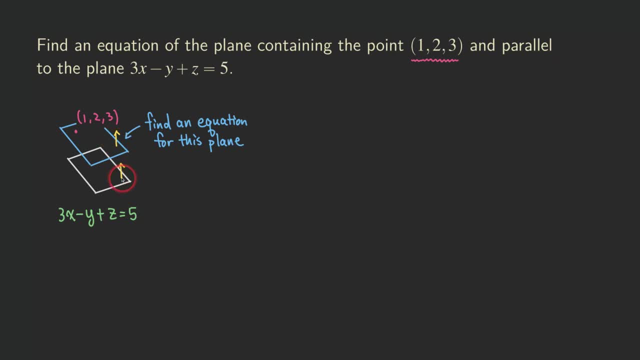 blue plane and then the one for the white plane. those two vectors are parallel to each other. In fact, we can actually use the same normal vector for the for the given plane for the plane that we want. Okay, so in this case we can already claim the normal vector for the plane that we're trying. 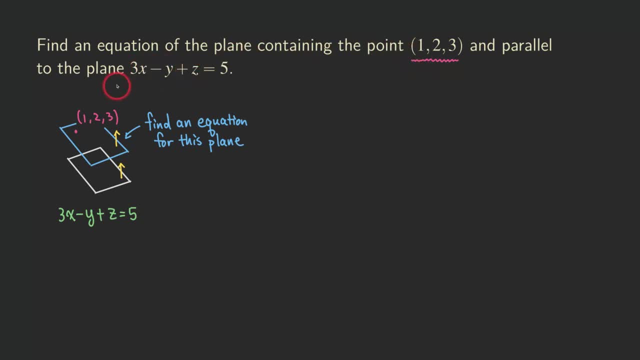 to determine would be the coefficients of the x, y, z that you have right here for this given plane. Okay, so let's just write down the information, So it will be easy for us to figure out the equation. So now, what happened is that we need a point. okay. 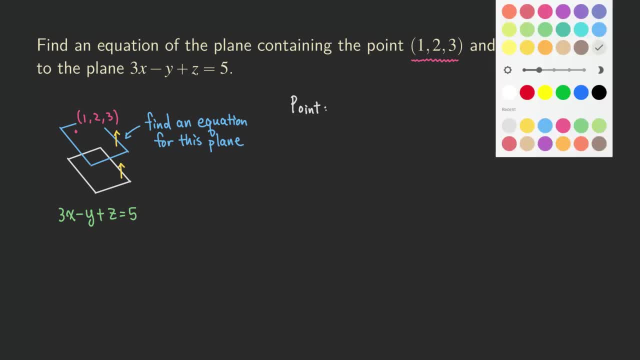 So first we need a point. the point is already there, which is what it's already given, which is one, two and three. Okay, so that's given already. The other thing that we need is the normal vector right of the plane, And so what is that? that's actually the same value that we have here. 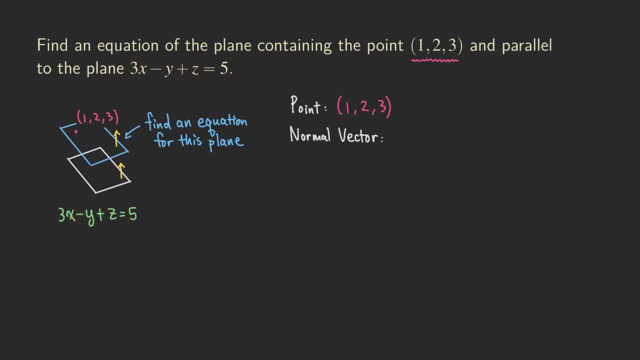 the normal vector for this green plane is. I mean for this, the plane in white right is actually what is actually. let's just write it down: it's actually just the coefficients of the x, y, z. So we have the three. 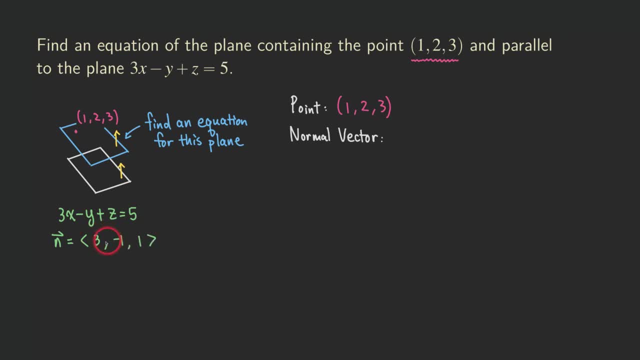 negative one and then one. In fact, you can actually use any, any scalar multiple of this and use that as the normal vector for the plane that we're trying to determine here. Okay, but right now let's just keep things simple. we are just going to use that same vector. 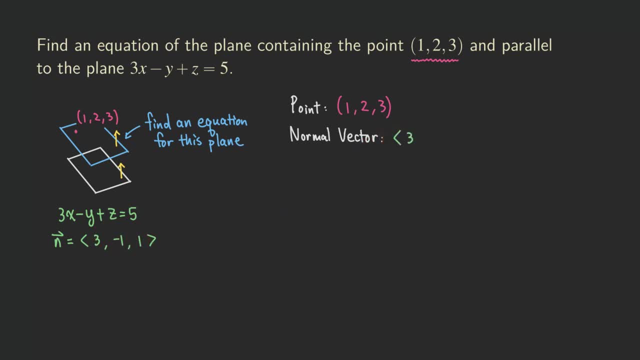 Okay, which in this case would be the three negative, one and one. Okay, so now we have all we need to figure out the equation for the plane. So right now, let's write down the equation. Okay, So now let's write down the equation. 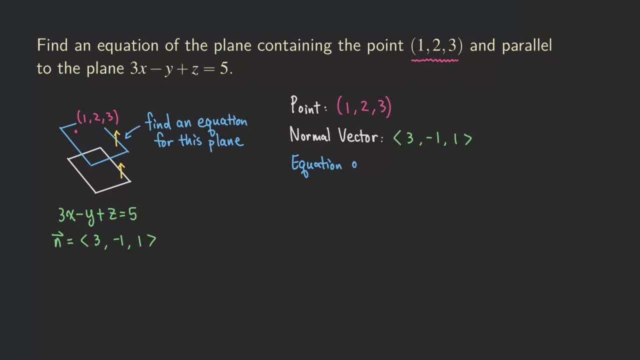 of the plane. And so how do we find this? We're going to use this. we're going to have the, the formula which is, or the equation that is, a, and then x minus x, naught plus b times y minus y. 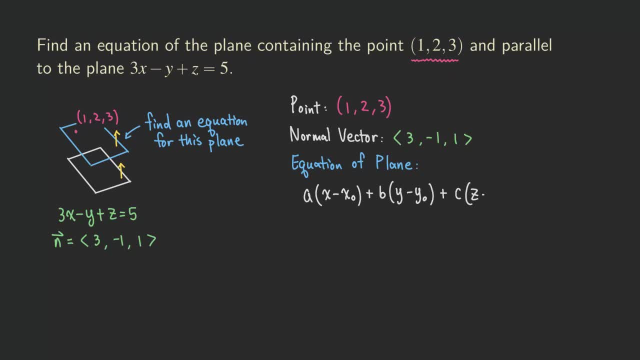 naught, and then plus c times z, minus z, naught right, and then that's equal to zero. Okay so the ABCs are actually the coefficients of the x, y and z And they actually come from the normal vectors. Okay so the A is the x component, the normal vector B is the y component and then the 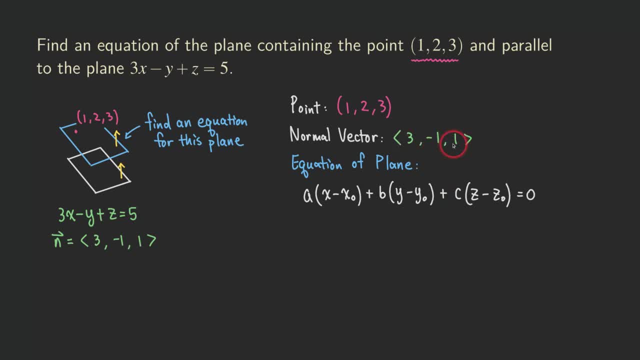 X is the y component, and then c is the z component of the normal vector, And then the x naught, y naught and z naught would be the xyz values of the point. Okay, so let's substitute those things. 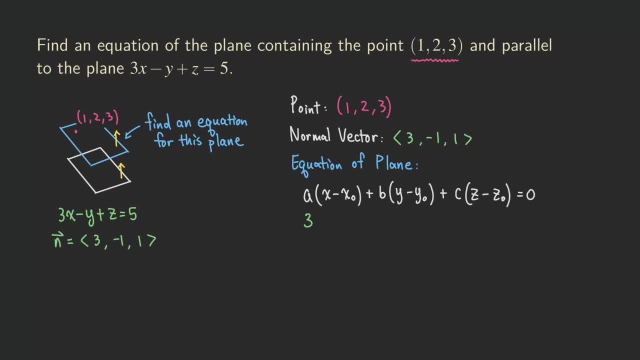 in there, then we are going to be getting the v, okay. then we have x minus x minus one, and then now minus, okay, minus the b. right b is here, So minus 1, and then you have y minus 2,, okay, which comes from the y value of the point. 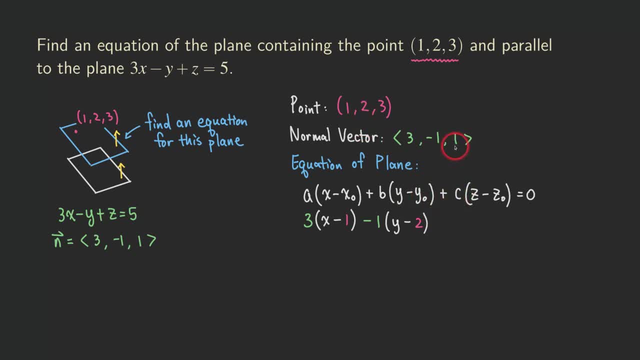 and then continuing with the c's, the c is the 1, right in the z value of the normal vector. so we are going to get plus 1, right, and then we have z minus. what is the c naught? c naught is: 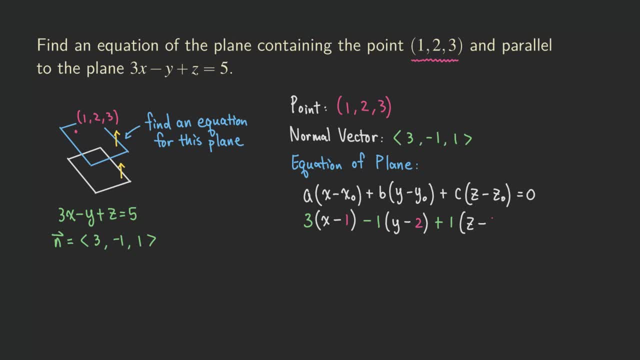 the z value of the point. so you get 3, right, okay, so now we have the plane equation. basically we're done, right, but we. if you want to simplify, you can do that too by distributing the 3, the. 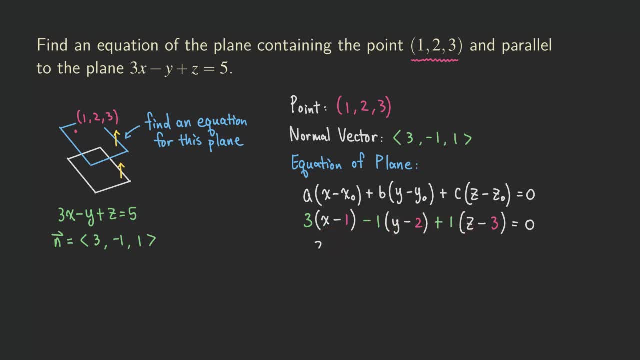 negative 1, and then the 1, so we can do that. if we do that, then we are going to get 3x minus 3, minus y, plus 2, plus z minus 3 is equal to 0, so now, if you move all those constant turns to the 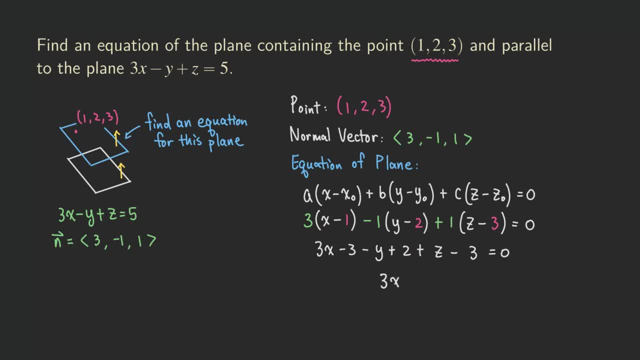 other side of the equation, then you get the equation to be 3x minus y plus z. okay, and that's equal to. what that's equal to if you move the negative 3 plus 2 minus 3, let's calculate that. 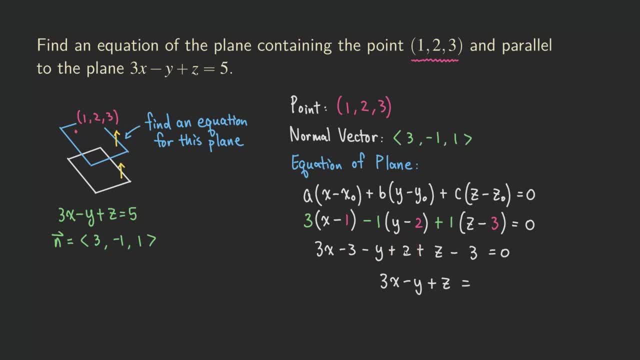 here that's 3, that's negative 3 plus 2, which is negative 1, right negative 1 minus 3, negative 4, and then it's negative 4 on the left side of the equation. so if you move it to the other side, 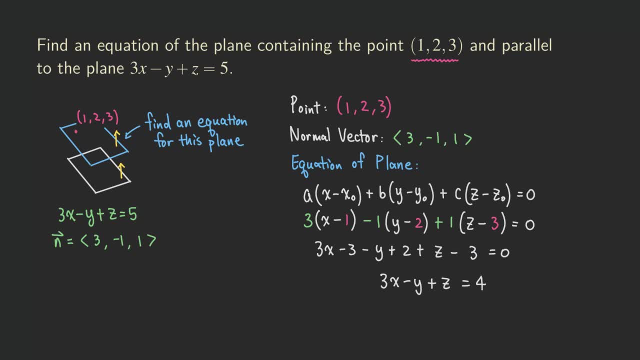 of the equation, you get positive 4, so now you have the answer for that one, And this is the equation, the plane that we're trying to find. so let me just highlight the color in blue, so you know that that's the one that we're trying to find here. okay, so, as you, 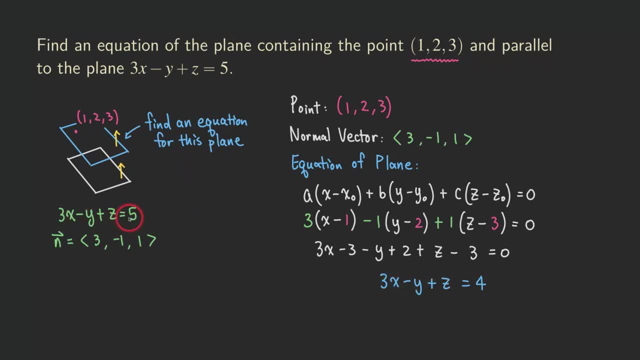 can see, the coefficients for the x, y, z are the same as that equation, except that the constant is different because that's a different plane. and so that you can see that those two equations- right, they have the same x, y and z coefficients, but constant turns are different. okay, so 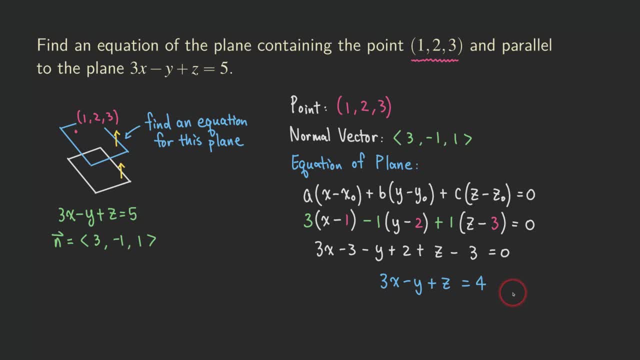 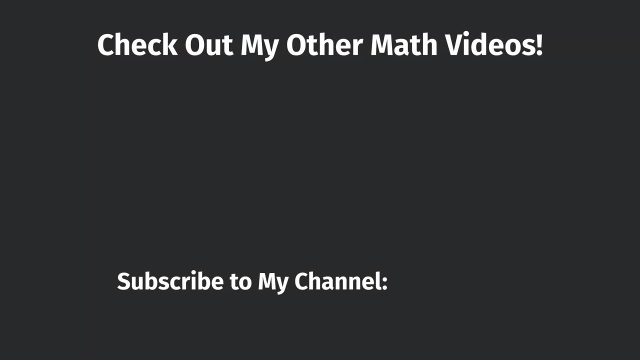 we can say that they're parallel. okay, so that's it for this problem. To help me make math learning available to everyone, please share my videos to others and subscribe my channel. it will give me support to make more videos. Let's work together to help. 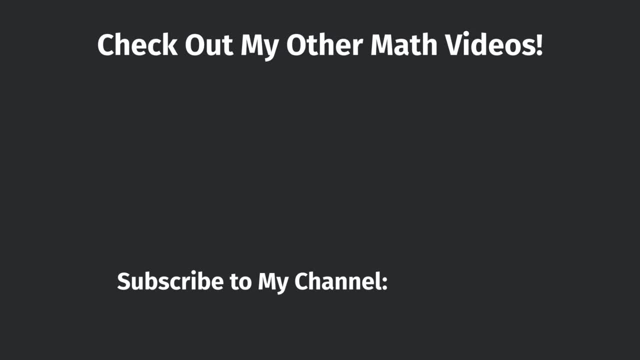 students and children learn math more easily. Thank you for watching this video.